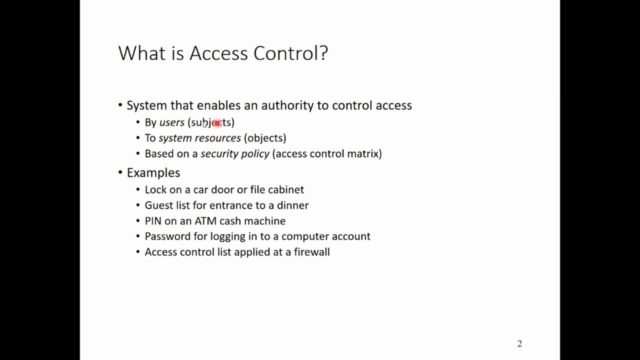 It might be accessing any other resources. So we have a set of users and set of resources, and then we have the security policy, which means how these users should interact with these resources, And we will see in a bit an access control matrix where you can define. 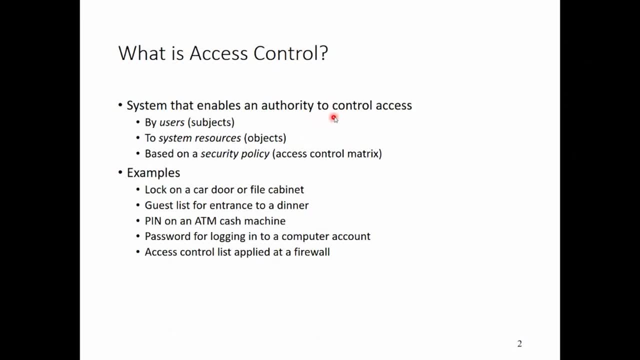 user x carried or write or delete some file from a resource or from a system resource. This is mainly the general idea or the general definition of access control And, to be honest, network access control is, let's say, controlling the access at the edge. 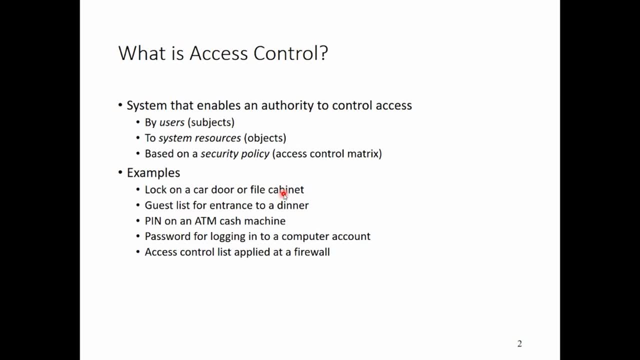 of the network. So it's the first thing of the network. It allows everybody who want to connect with our network to follow the network policy. And let's say, if you have a Wi-Fi network at your home and if somebody stop at your door and connect on your Wi-Fi, 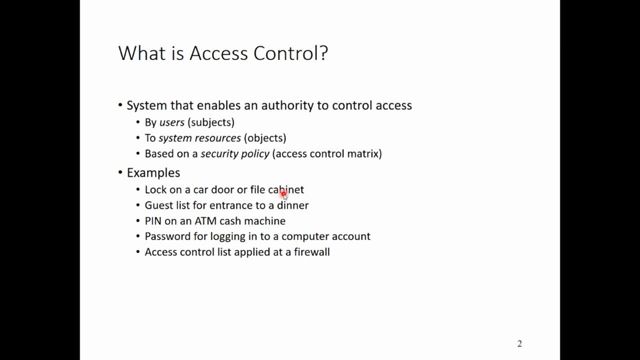 so you need a policy to let that person connect on the network or prevent or prohibit that person from connecting on your network. And sometimes this kind of policy is not really written, It's a technique, For example, at your home using an encryption wireless network. So if that guest or that user at your door 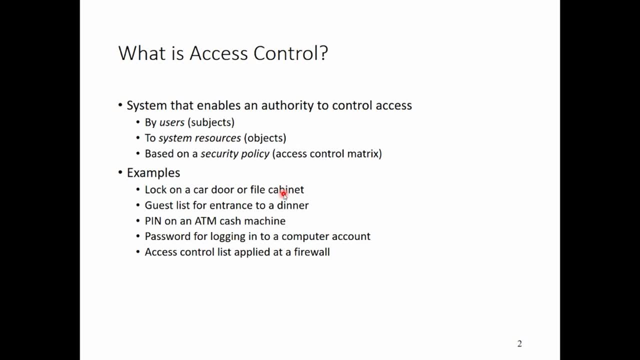 does not have your encryption key, that means he does not connect at your network And some kind also of network access control is to perform a health check. Health check means is that device you want to connect at, let's say, our university, is a trusted 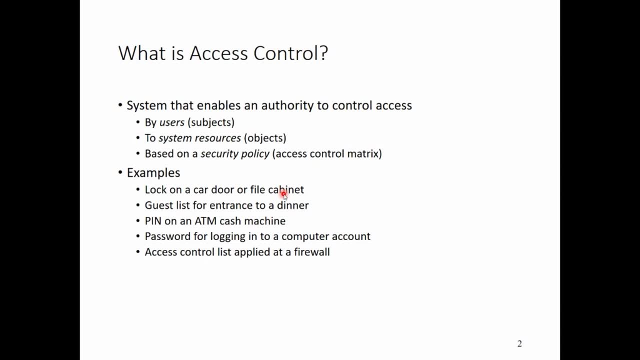 university. So if that device has an antivirus on it, is the antivirus, for example, updated Or is the antivirus software is the recommended one, or recommended by the university? for example, Is this device belongs to an employee or a student at the university? 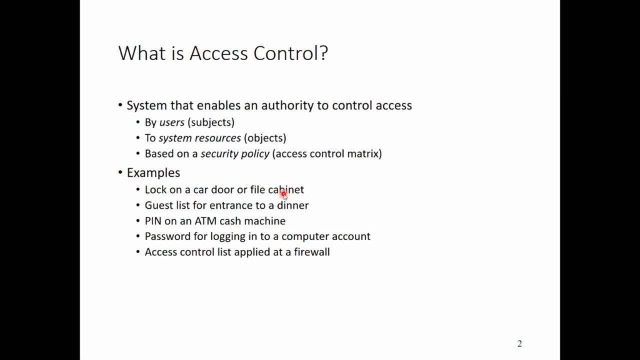 or something like this: Is it a mobile device or a laptop, or does it use Windows, And is the Windows updated, or the Mac OS, and so on? So all of these healthy check is defined as an access control. So there are many examples on access controls, right? So access control. 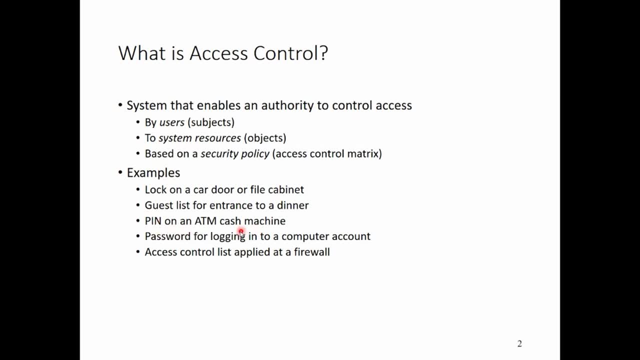 for example, the pen on ATM, cash machine or ATM cards is an access control. The password is an access control. The access control list which define at the firewall of course, which define who can access what is an access control? To lock your door or to lock a file cabinet is an 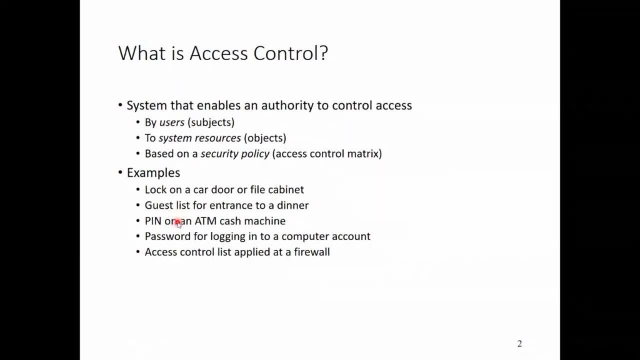 access control. So you need a card or a key to access that file cabinet. That's an access control. A guest list- who can enter for a dinner party or something- is an access control as well. Right, So this is mainly the definition. 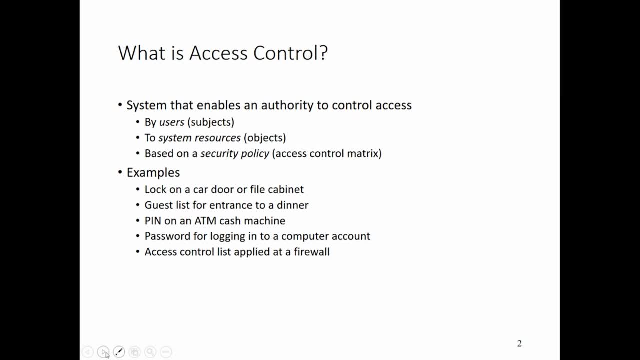 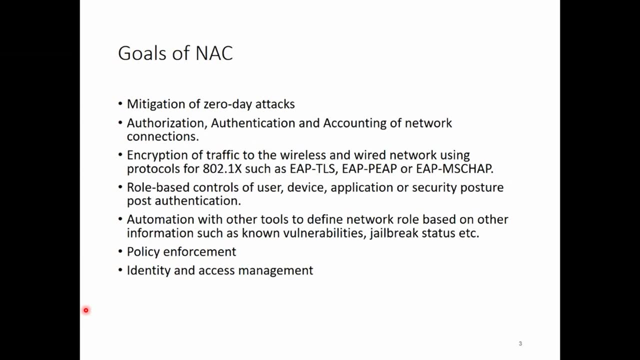 The definition of network access control. But I want to ask in general: why do you think network access control has appeared in network security? True, To protect our network from any malicious, let's say unauthorized, user, And to protect your network. That's true. 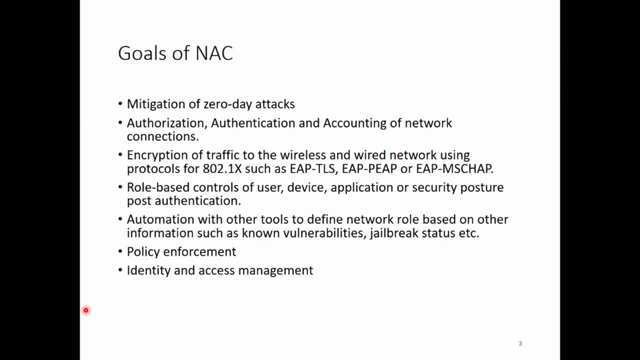 So to protect any kind of network, to protect who can access what, as network access control is needed. So imagine that you are in a journey and you are at some hotels and you want to access the hotel Wi-Fi. So if the network does not recognize who are you and what are you doing? 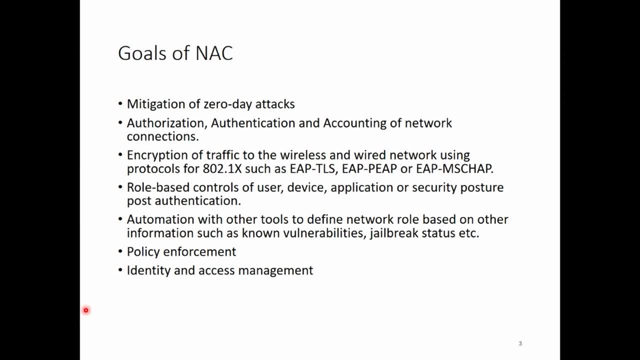 so they will not allow you to access the network And I was looking for a robot answer because access control maybe increased And the need of access control solution increased after getting wireless network and after getting wireless devices and mobile devices as well, So you can't know who is the user of this device. 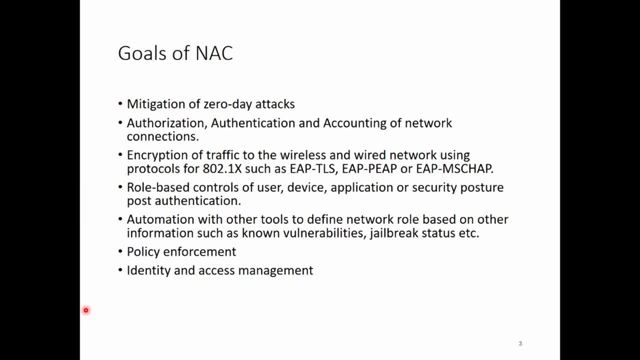 because of the many devices that are requesting to access the network. To be honest, we will talk about VLAN maybe in the nap, but I will just draw a symbol here. And do you know that the network switch has many ports on it And one of the main network 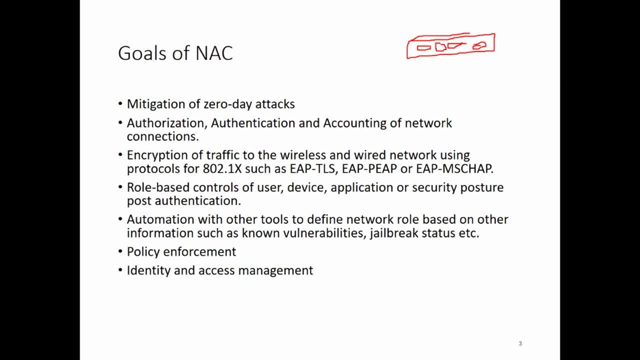 access control is called IEEE 802.1x, 802.1x, And that technique is, which is which is PNAC, Port Based Network Access Control, Which define that, for example, if we have these four ports, two of them are belongs. 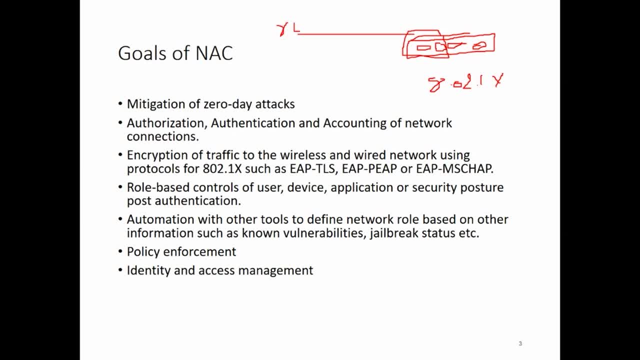 let's say to the VLAN one, which is the accounting department, for example. So if any PCs are linked to this port can access all the other devices linked to the same VLAN, While they can't access the other VLANs on the switch. So during this VLANs, only the allowed devices can access the. 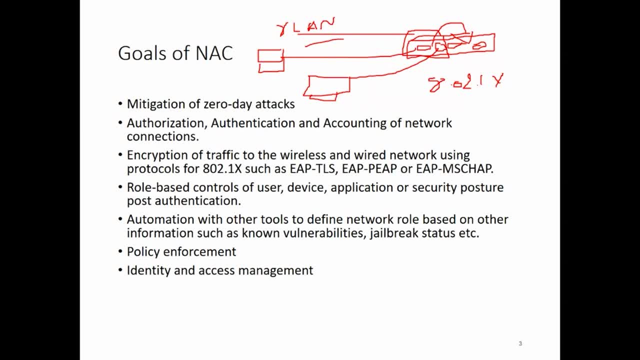 accounting VLAN, And we have many kind of VLANs. We have, let's say, VLANs in the same geographical place, which is as the 802.1x, the port based network access control, and we have also the virtual private area, the VPN, as well, Which are to connect two different locations. 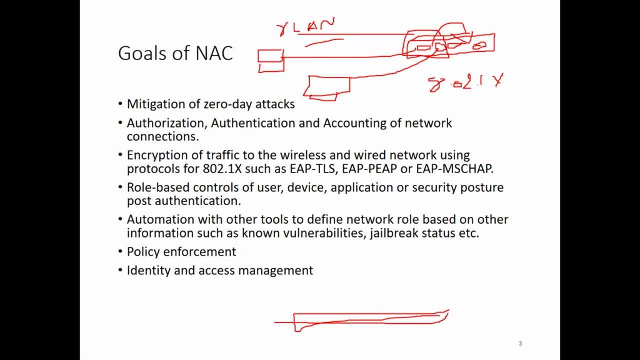 through tunneling process or through the internet with two different geographical location and to let these devices access, as they are in the same line. But we need to explain them together. so the first one is mitigation of zero-day attack, and it's clear that if we have a network access control then we are preventing any 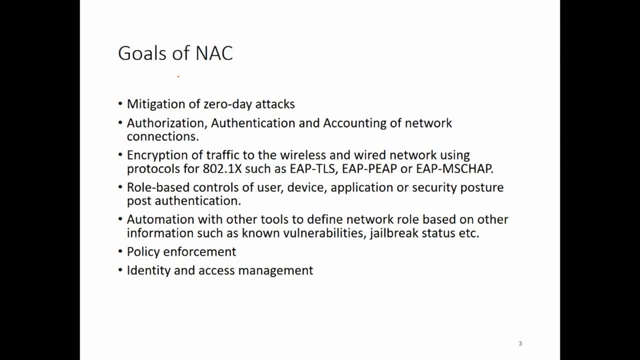 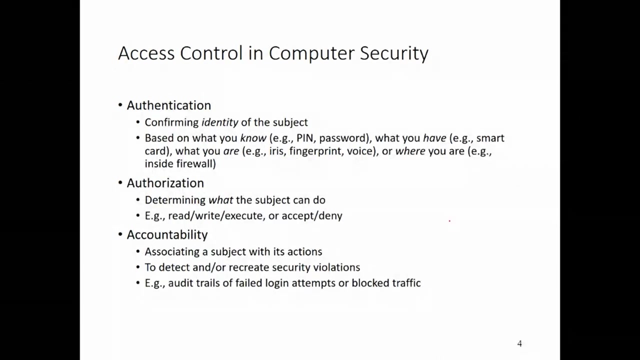 unauthorized PCs or any unauthorized user from getting their access to our network, and that will really reduce the number of attacks and mitigate any zero-day attacks also. the second goal is to give authorization, authentication and accounting and in a bit, in the second slide and third slide, for sorry, we will. 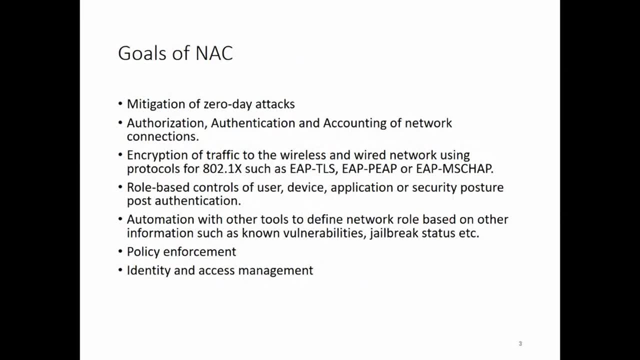 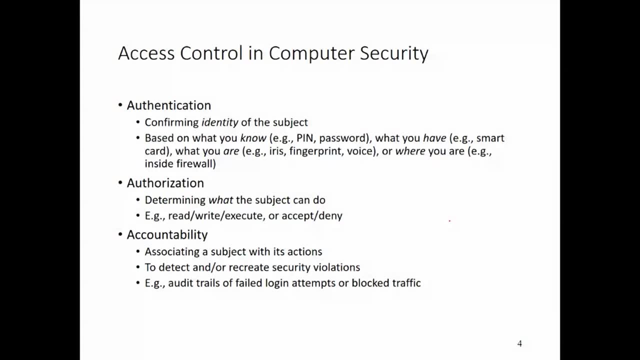 see what. what's the main definition of authentication, authorization, and why not do it now before continuing the goal? so, authentic, what's the difference between authentication, authorize a or authorization, authentication and accounting? so authentication may mainly as to to let the network know who is accessing this network. so if X want to access this, 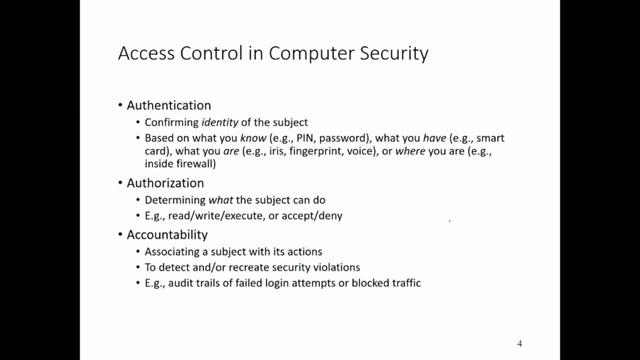 network. so the network should make sure that the entity who want to access this network is the one who claimed. so if Hisham want to access this network, so the network should provide some mechanism to let Hisham prove that he is Hisham, or by 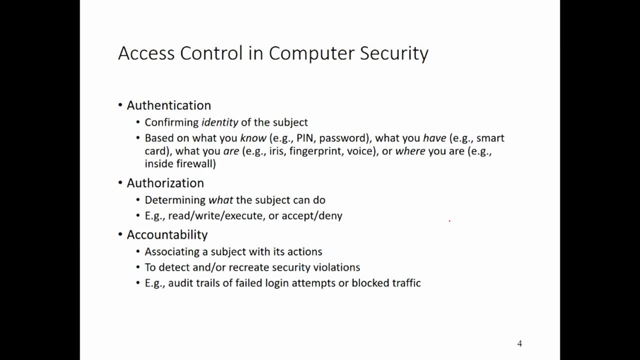 using password, pen, fingerprint, whatever accessible in the network, and these kind of authentication it's called a service that the network should provide and network should provide a mechanism to to identify identity of any entity want to access the network. so, for example, most of us, when we are using a, 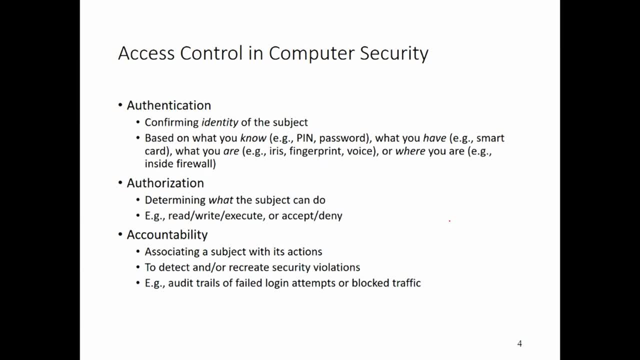 the university wireless, we should provide our ID and password and that's as an authentication technique. we have to have an authorization. authorization means something different. authorization means the privilege that you have. so some user they might have, for example, on the e-learning system, some user they have. 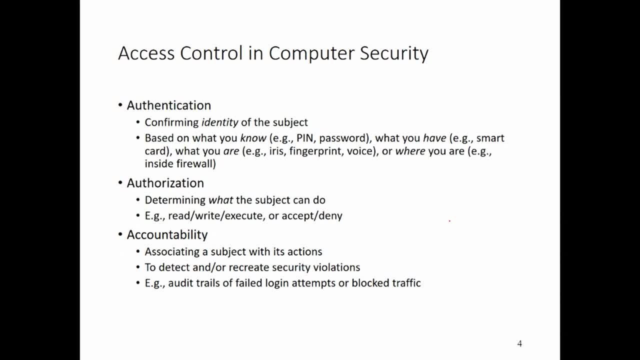 only to read from that e-learning system and, let's say, an instructor and staff, they can modify marks, grades, upload material presentation, etc. so authorization means to determine the privilege of the user on the system and that's what, determining what the subject can do. so and the last one, which is accountability, and mainly accountability is to measure. 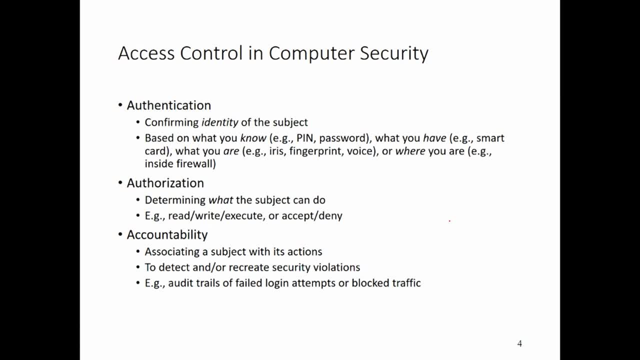 to measure all the traffic and that's really. it's like a look file that you have to record every single access and every single request and response in the network, and this is accountability. it might be used also for billing system, especially in the cloud infrastructure, and also it can be used 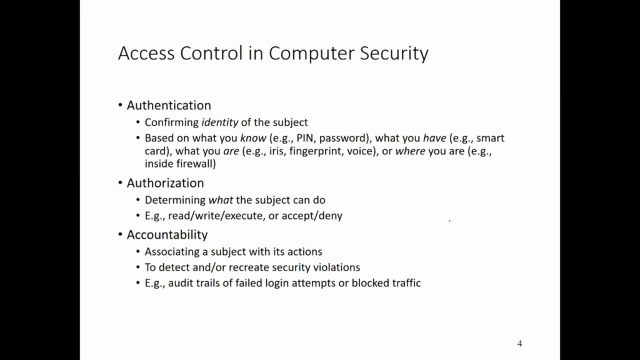 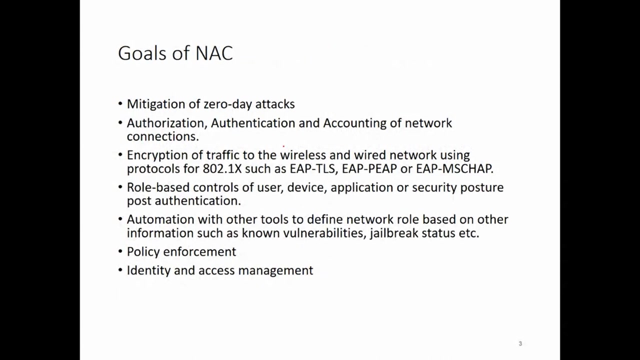 as I guess one mentioned, for crime detection and so on, when we go back to all the history and look like who accessed our news network and when, and what they have done and so on. so this is three is of access control, which is called authentication, authorization, accountability. the third: 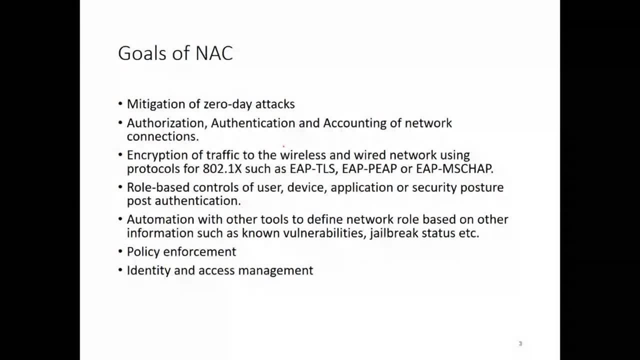 goal of network access control is to encryption of traffic, especially to the wireless network, and also it can be used also in the wires, in the wired network and in the wired network. we we usually use the 802 point 1 X, which is the port based Network access control, as we explained before. also we we can use the. 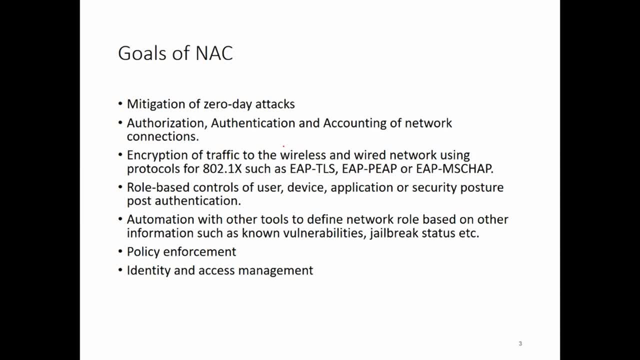 network access control to define the role based, which means each user and the role of that user on every device, on every process, on every application in the network. and that is a role-based control. and we normally use that role-based control to detect any intrusion in the network, so we can use network access control to support the intrusion. 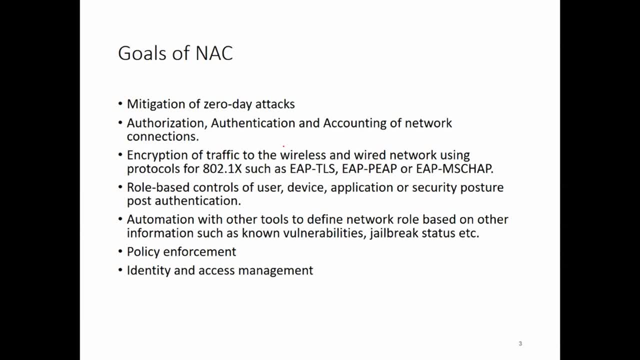 detection system and also to identify the malicious, let's say or that users who can be intruder, and sometimes having more than one security solution in the network, they support each other also. the other goal of having a NAC or network access control solution is the automation. 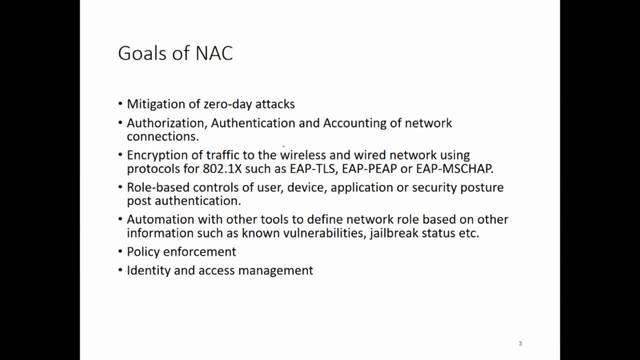 process of define the network role, and this means that we can have an automated process to define any jailbreak or any threats or any vulnerability inside the network. having network access control also means that we have one policy and that policy should be followed by everybody, and this is called policy enforcement. enforcement means that you define 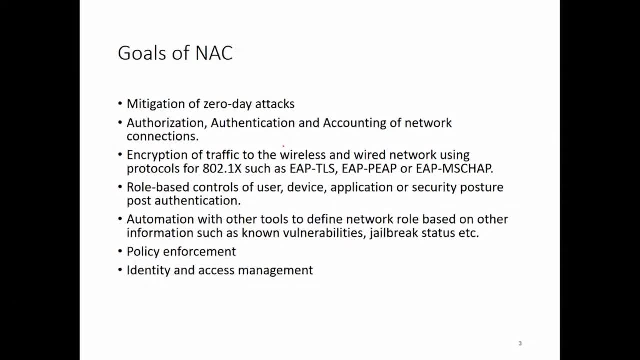 a policy that everybody, every computer, every user accessed your network, should allow their PCs or their laptops or their devices to follow that policy from the moment they accept to be connected to your switches or to your router or for your, to your network with their boxes. so that means a policy enforcement and also the other goal of having network access control is 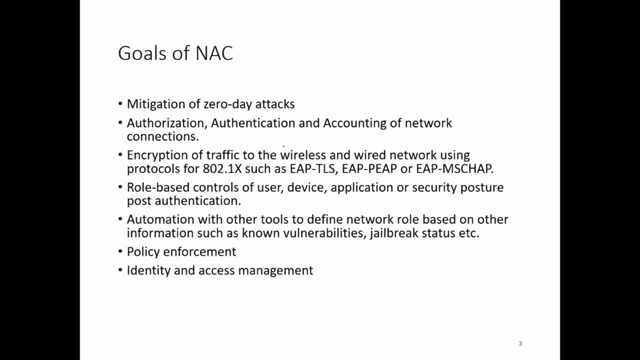 to identity and access management, which means that sometimes you are giving an IP address to a new and user, to a user who are not recognized for you. that's why having a network access control will let you know who's accessing this IP addressing or who's accessing your. 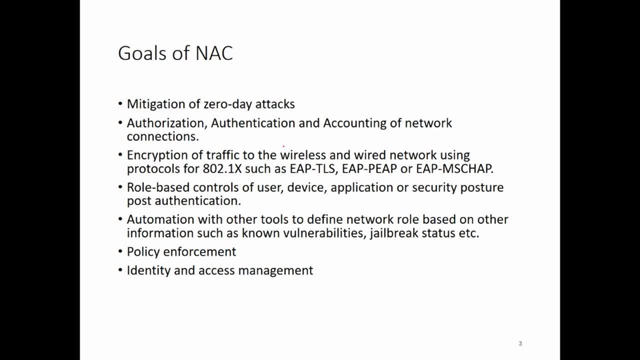 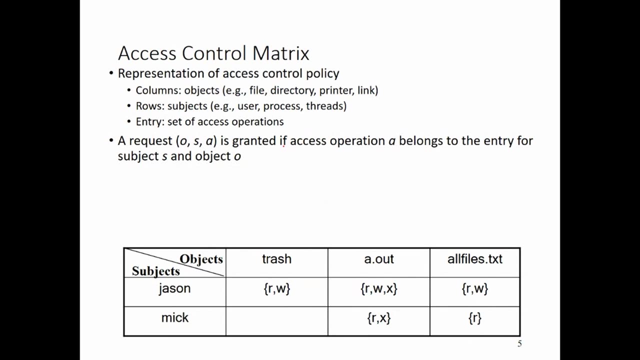 network by this IP address or who is the authenticated user identity inside your network, which is very important for all kind of network. okay, guys, so this is mainly access control matrix, which we described before, and this is the access control matrix which we described before, and this is the access control matrix which we described. 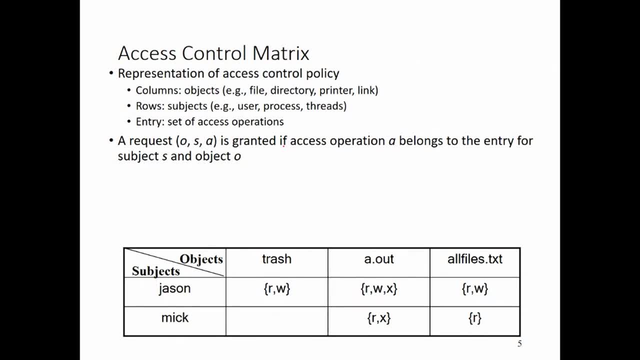 before and this is the access control matrix which we described before. the columns which- yeah, the columns which are the know, the columns which are the object and the rules are the subject. so the object means any process, any resource. you have it inside your network. so, for example, you have this access control. it's not really for a network, it's. 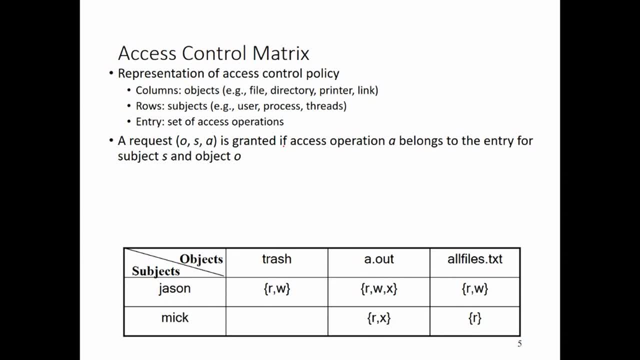 a for operating system. so, for example, who can access the file in the trash? who can access the file edit out, who can access all text files? and we have two subjects or two users or two entities- Jason and Mike- and we are defining a set of entries. this set define the access operation. for example, we have 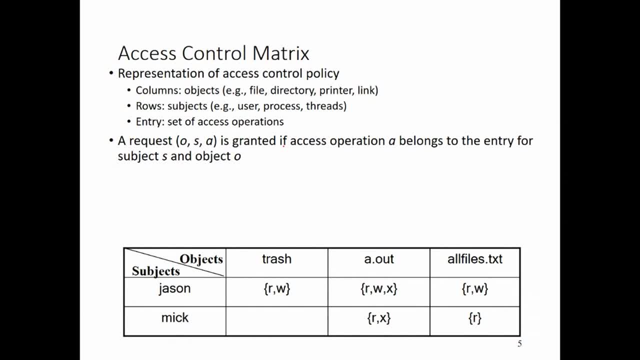 read and write, and X, which means delete. so this kind of access control matrix might be used on the firewall, called user permission. it is yes, it is your user permission. you can define this user permission per file or you can define it per system. so if you define it per file, it's a user. 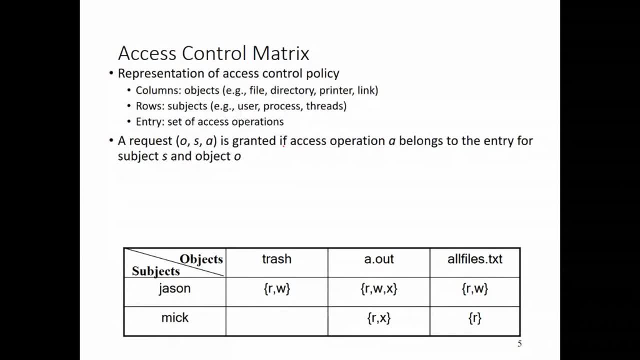 privilege, but if it, or permission, if you define it per system, access control matrix, or sometimes they call it access control list: yes, x is execute, true and r is read and w is right, and you can define any other kind of operation as well. all right, two implementation. 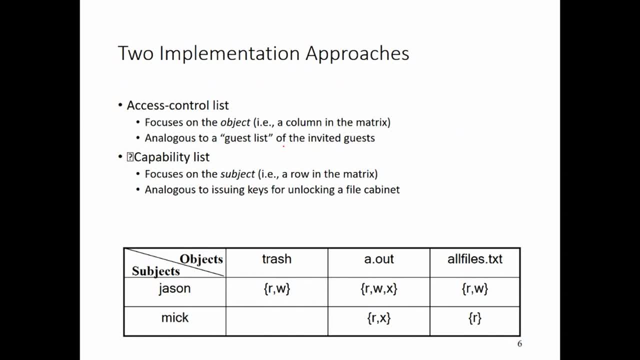 approach for access control list and capabilities. but before talking about access control list and capabilities, paul has mentioned in his video that we have two concepts for defining network access control: the pre-admission and the post-admission. what do you think the main difference by the pre-admission and the post-admission? it's a true revealing design. 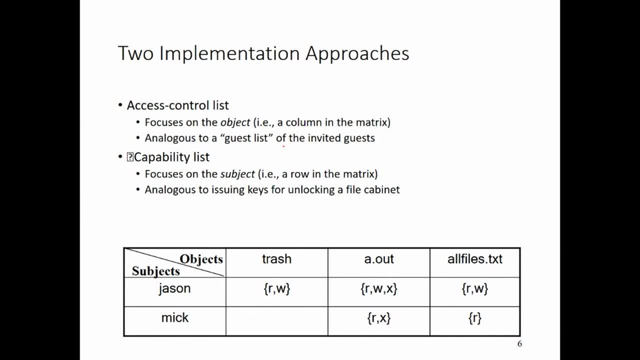 in knack. yeah, but i want to uh. yeah, but i want to just add on that. for example, if we have a client who want to access our network and that client, for example, has uh- uh out of date and virus, or has an uh- an updated uh operating system, so we prevent that client from accessing our network until they 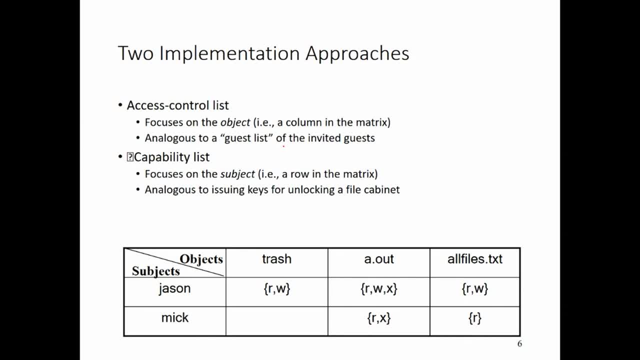 have uh uh everything updated while the post. this is called a pre-admission. why the post admission? mainly is to uh uh uh, follow up on uh all the user after getting uh uh their access to our network and then, based on their, let's say, actions on the network, we can have a further decision on for enforcing them. 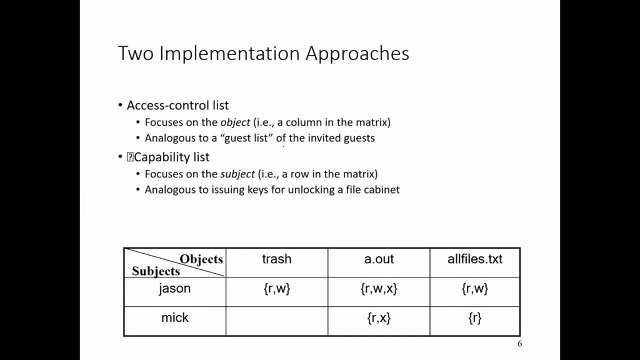 to disconnect or enforcing them to follow some policies that we are defining in the network and that policy should be followed. so basically, as guy said, pre-admission is to uh control who can access before uh their access to the network, while post admission is to uh uh follow up with the user. 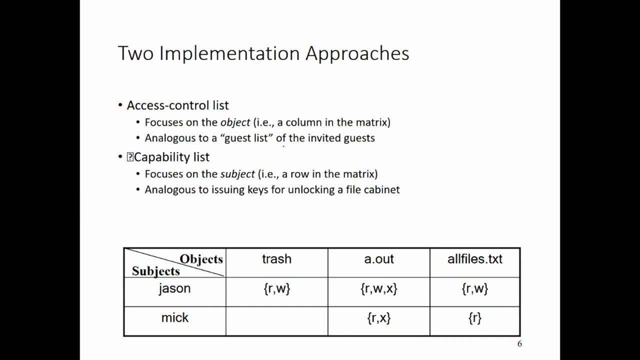 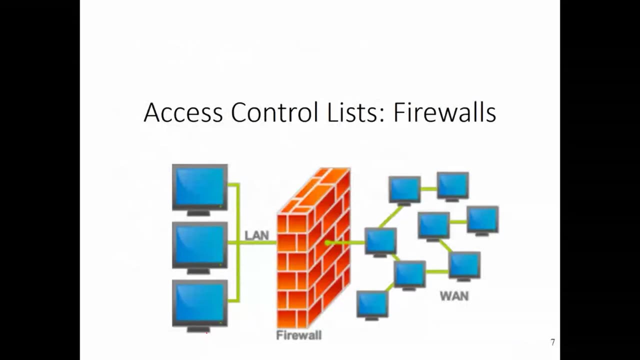 after accessing the network and see what they are do, uh, what they are doing in the network and what action they have done. that's right. and also paul mentioned, because, uh, these stuff are not mentioned in the in the slide here. that's why i want to focus on them, uh, uh, also paul mentioned that 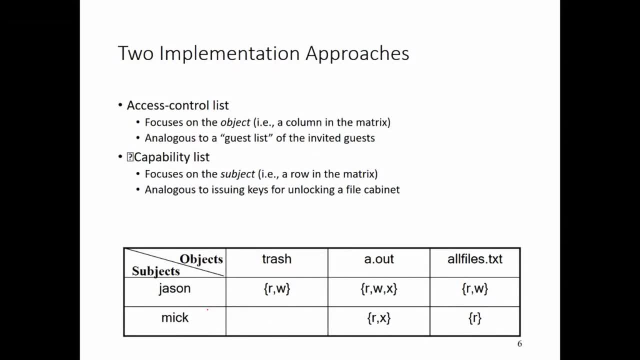 we have two fundamental uh uh ideas behind uh network access control: the agent and the agent less network access control. i wanted somebody else, rather than guys, to let me to let me know what they think uh the difference between the agent and the agent-less network access control. 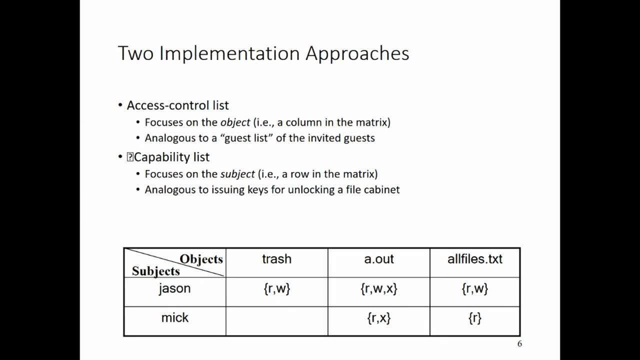 true, so agent network access control. they are using an agent software and they require an agent software. so, for example, you have an agent, uh, for google drive here, right? so if you, if you don't have an agent for google drive, you can't access the google drive. 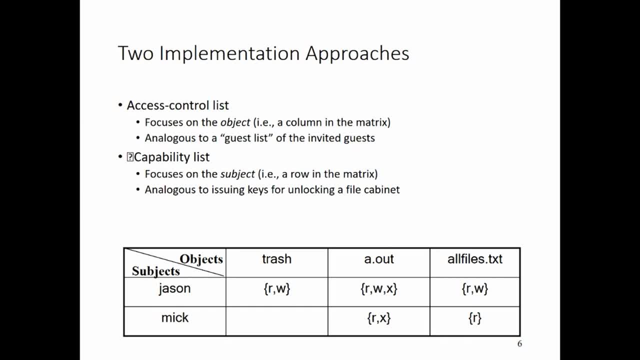 itself and other kind of network. they provide you with the agent software that you have to download, and some hotels as well, they provide you with their application that you have to download in order to connect to their wi-fi, and this is called agent software- network access control, while the other kind of network access control, which are called 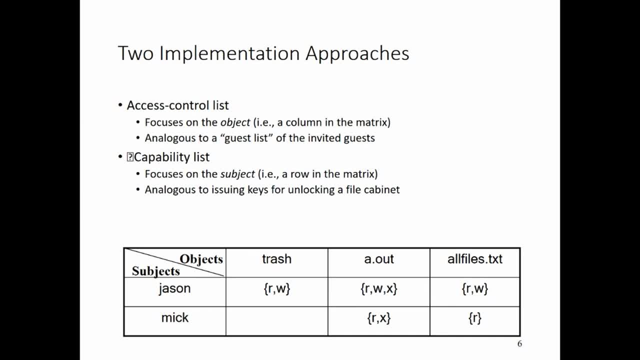 agentless. they do not provide you with any required software to be downloaded on your machine, but they use scanning systems and scanning solution to find any network uh inventory techniques and to detect any discern characteristics uh remotely by the network itself. so this is mainly the difference between agent and agent-less. 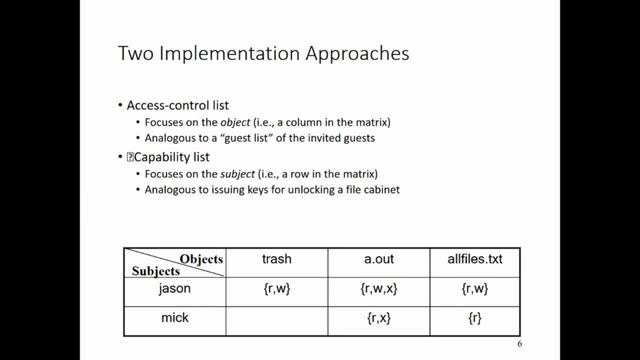 access control. one of the famous agent network access agent, is called network access protection and this network access protection is an agent to the windows uh server and it's included in many versions of windows 7, vesta, xp and other other linux as well. very versions, all right, okay, so let's follow up on uh two definition: access. 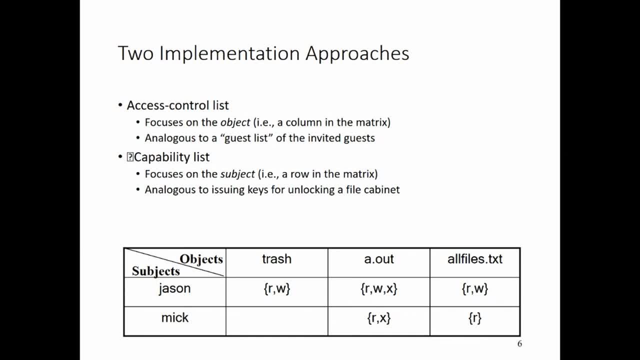 control and capability list. uh, we will come in a bit about the difference between uh access control and capability. but mainly access control is to know is accessed by who and what's the operation that can be performed on that object. why the capability list is focused on that. who can use these? 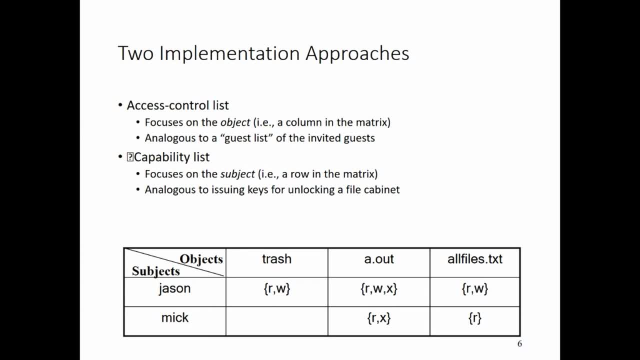 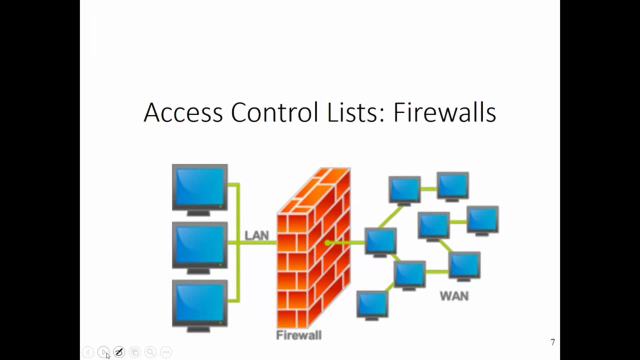 resources or not, right, okay, so, as we mentioned, the main, let's say access control, is provided by the firewall and we have, and we have many kinds of firewall and, as you see here, a firewall it is something between your local area network and the one, or the wide area network or the wireless, not the 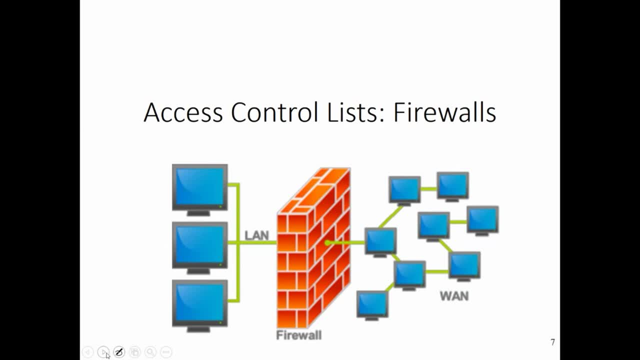 wireless, the wide area network and mainly, if we can define, a firewall. a firewall is a control that is controlled by the firewall and we have, like a bottleneck: who check all the packets come to your network and who check all the packets going out from your network? we have many different type. 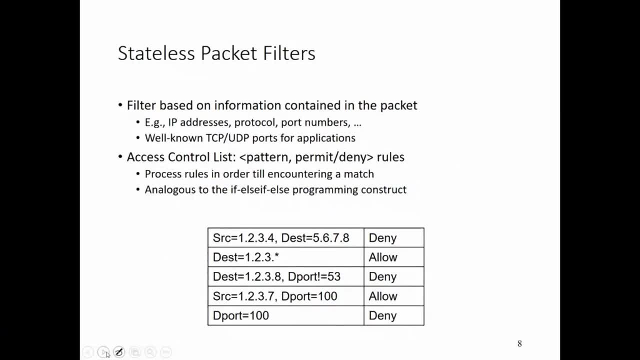 of firewall, the first of which is stateless packet filter, set this packet filter which define the rules of the packets who can pass through this firewall, based on the IP addresses and the protocol is used and the port number, without looking into the packet content itself and without 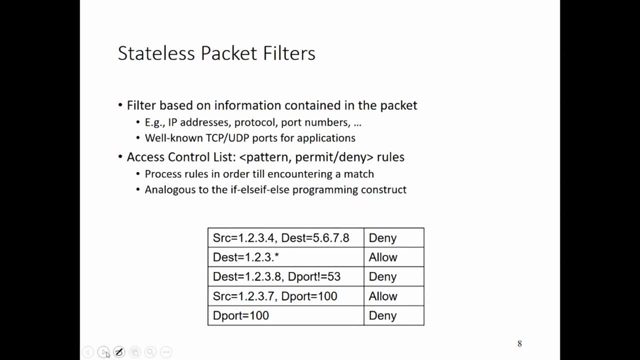 controlling the data inside these packets. so the the state for- sorry, the stateless packet filter. it's only giving access based on the source IP, the destination IP. for example, you can see in the table below here that we have a certain source. they can't talk with a certain. 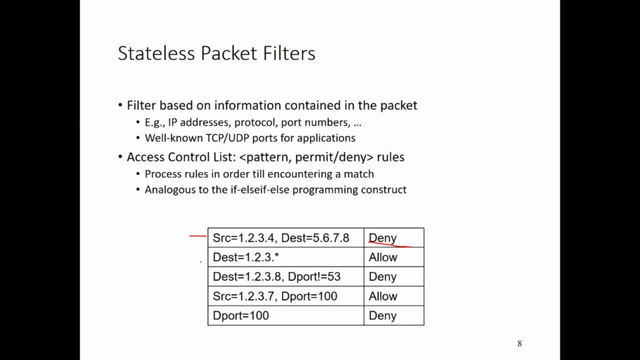 destination, because the action is denied, and the destination one, two, three, dot star, for example, if we can imagine this is an IP address, it's all allowed to be, let's say, contacted from our employee, for example, and in the third law, all the destination IP address one, two, three, point eight, on a certain port or in the 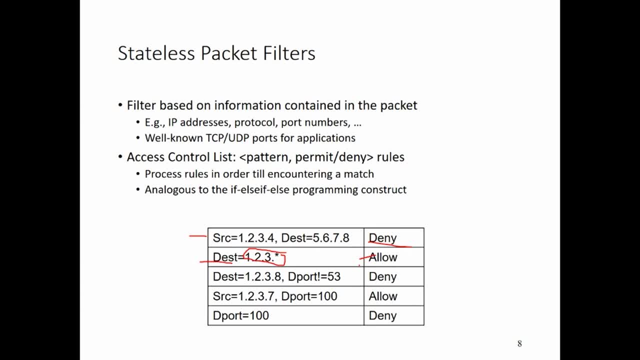 port not equal to 53 is denied. so this is only an example to let you know that the stateless packet filter- it's based on IP addresses, port numbers, right, and and the other kind of firewall, which is the stateful filter, which is also based on. 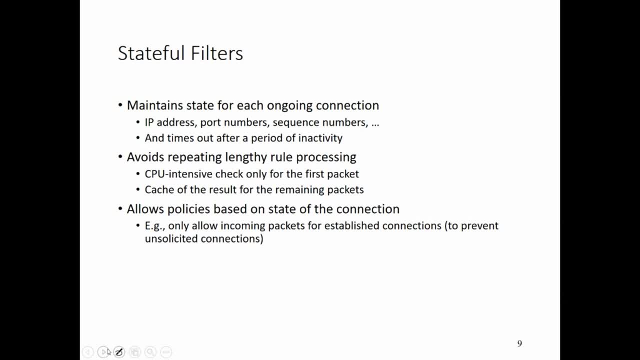 IP address, port number and also a sequence number. but it's the difference between a stateful filter firewall and state this filter firewall that we also examine the content of the packet. so we also look for the headers of the packet. we also look for the headers of the packet. so we also look for the headers of the packet. 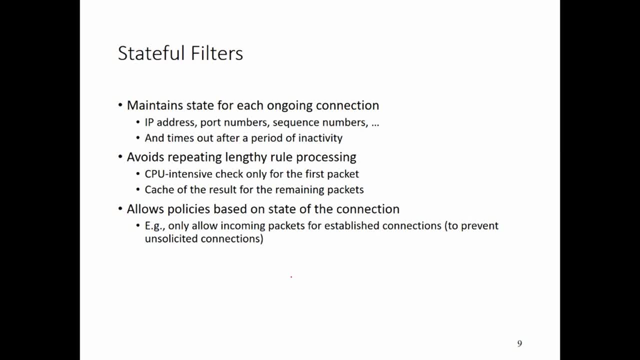 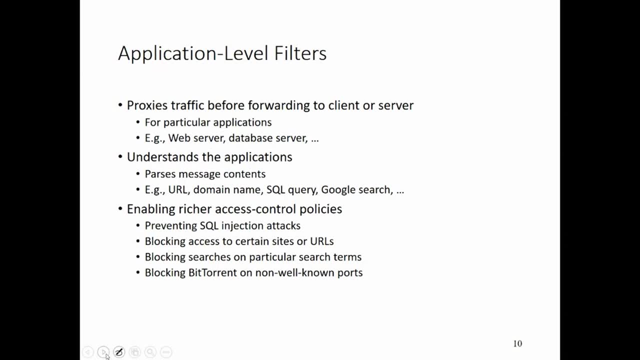 and then that filter filter. we can establish the connection based on what's inside these packets, right? the third type of the firewall is called application level filter firewall and sometimes they call it proxy firewall, because they examine the application used in the packet. so, for example, this a tcp packet or udb packet, based on the application layer protocol and 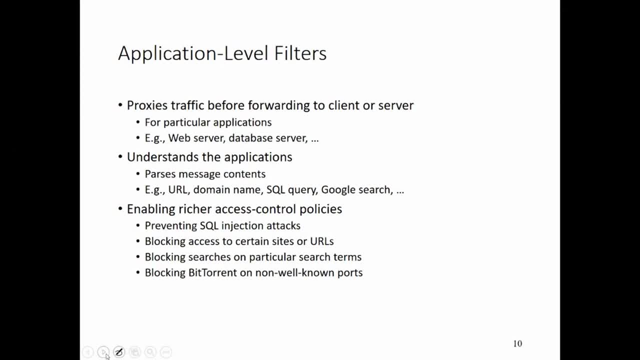 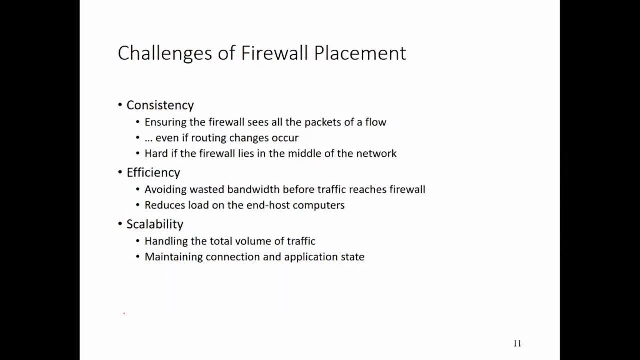 they, let's say, prevent any kind of malicious application to be accessed from outside or to be sent to our network. but all of these kind of firewall, to be honest, uh, has some challenges. one of these challenges is consistency. consistency means we need to place this firewall in a position that can see all the packets. 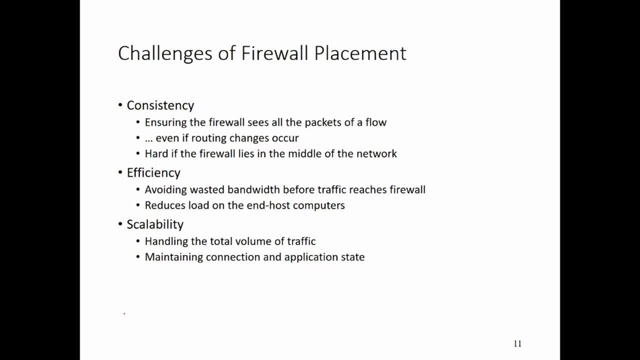 coming to our network or going out from our network. and also the other challenge that these firewalls should be efficient enough to avoid any bandwidth traffic and to avoid any congestion that they could provide to our network or they could make it in inside the network. and this firewall should be scalable enough to handle any kind of 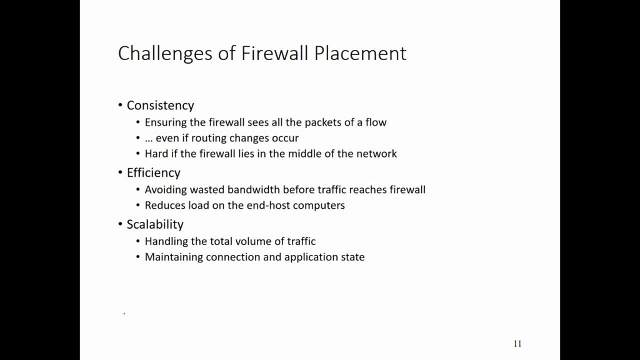 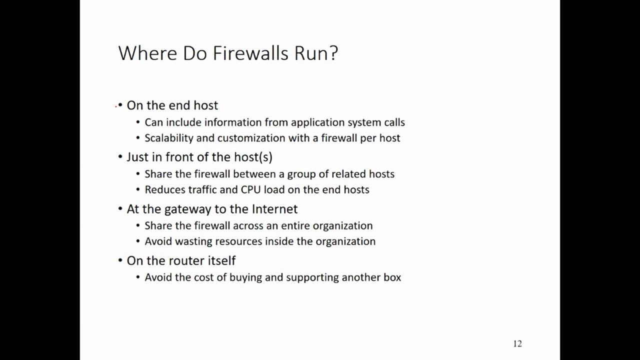 traffic, especially with a huge number of devices inside a local area network. the four also these firewall. they should be placed easier on the end host which means that just before the host and they can examine all the packet coming to a certain host or it can be in front of the host. 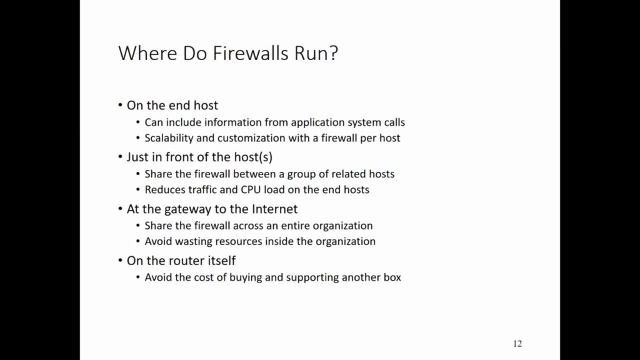 which means that it can be before the local area network, or it can be attached to the gateway to the internet, which means it's like the network access control at the edge of the network, and that means before going to the outside world, before going to the internet, or it could be a software. 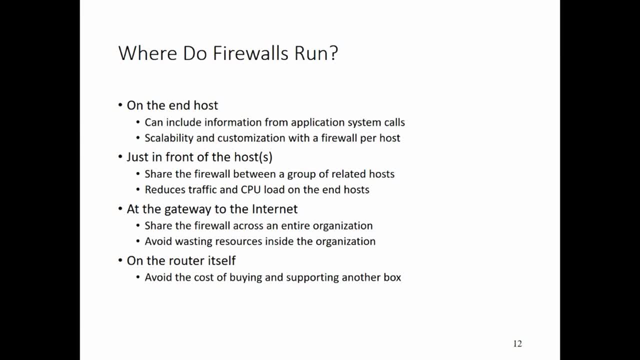 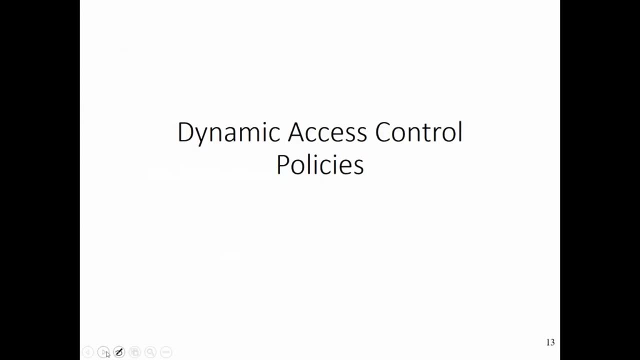 implemented on the router itself, right? so this is mainly a brief about a firewall, and we have also. we have also the other kind of access control. the first one was the, the matrix, the access control list or the access control matrix. the second kind is the dynamic access control and dynamic access. 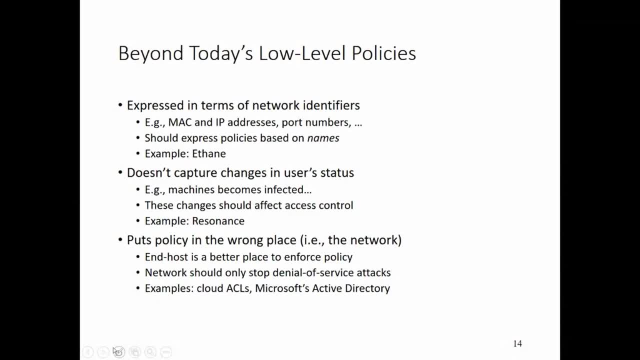 control is mainly based on defining a policy and it's called bring your device policy and or py. I will write it down here: py-listing-advice-policy. I will write it down here: py-listing-advice-policy, Bring your own device policy- BYOD, right, And this kind of policy is really very dynamic And an example of that is Ether architecture And also we're seeing a bit the dynamic algorithm to, or the dynamic protocol to detect any access. 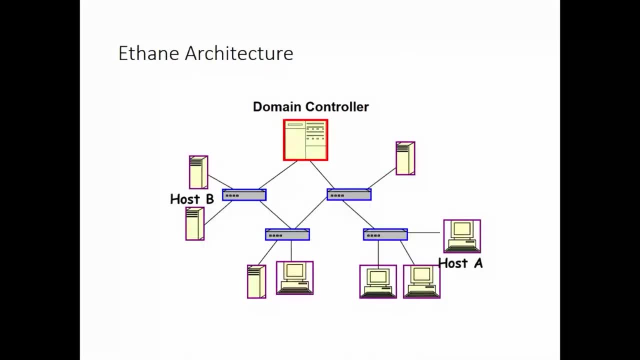 So, for example, if we have a domain controller and that domain controller are issuing the IP addresses for all the hosts which are connected in our local area network. So, for example, host A want to access the domain controller in order to get an IP address. 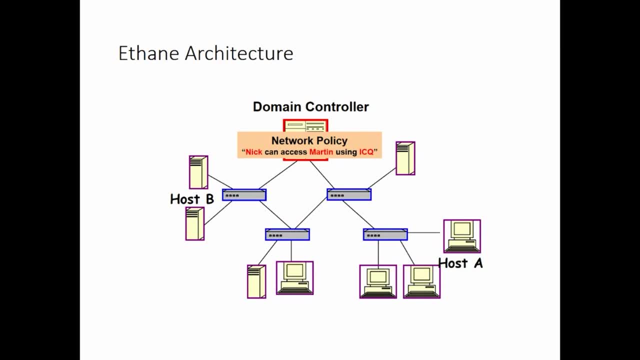 And in this example, If host A is Nick, for example, and host B is Martin And Nick want to access Martin and send ice cube messages, Let's see how host A or host B can get the IP addresses from the domain controller. 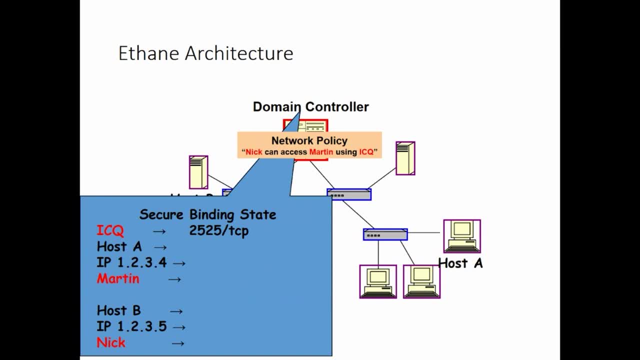 So host A, they define that they have a secure, binding state to the domain controller And they asked: controller: hi, I'm host A and they should provide an authentication technique, either a PIN number or a password. and then the domain controller and they 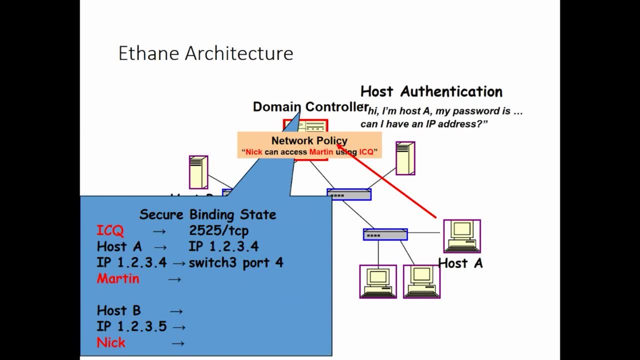 request an IP address, for sure, and then the remote control will define the IP address for host A and they let host A to be connected on switch 3 and port 4 and that's all accounted and saved in the log file in the domain controller. so 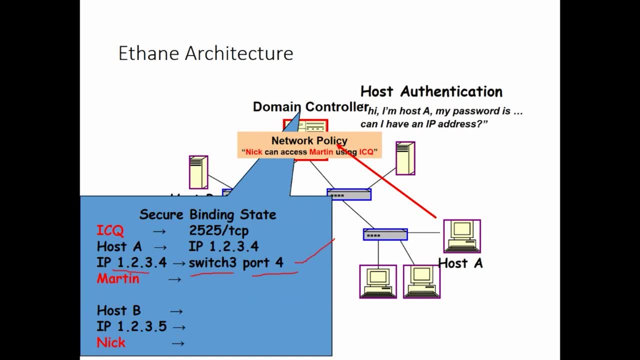 we know now that host A is connected on switch 3, port 4 and using this certain IP address and NIC, they have to do the same thing. so NIC is also sending a hi message to the domain controller asking to provide an IP, and the main controller makes the same purchases. thepler says: yes, we are sorry, we all know what is delineation in QUADARreceiver. They send a high message to the domain controller asking to provide an IP and the domain controller 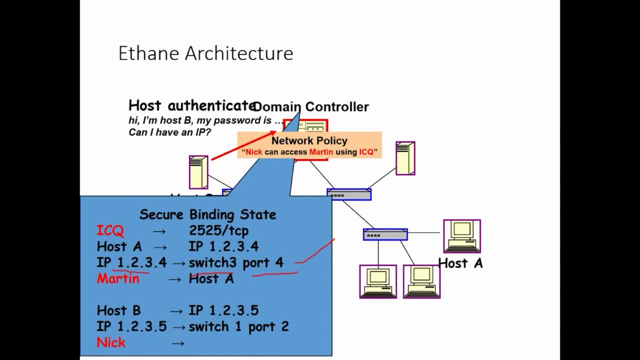 controller. after checking the password of Nick and getting B authenticated, they have to provide with an IP address, And now we know that host B is linked on switch number one and port number two And afterward they can use the network to send their messages between each of them. 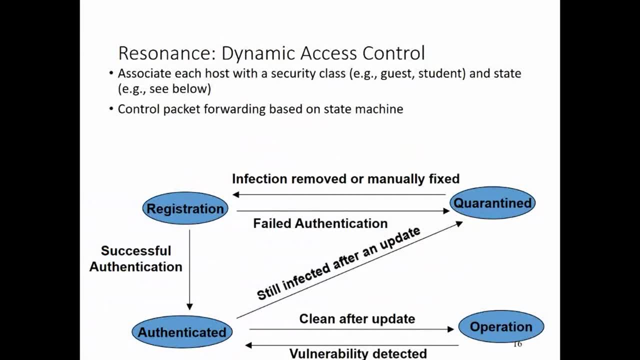 So this is ethon architecture And the other one is the dynamic access control, which basically means- excuse me, let me just focus on this and I will come back in a bit. So the dynamic access control means that we have four phases in each device want to access the network. 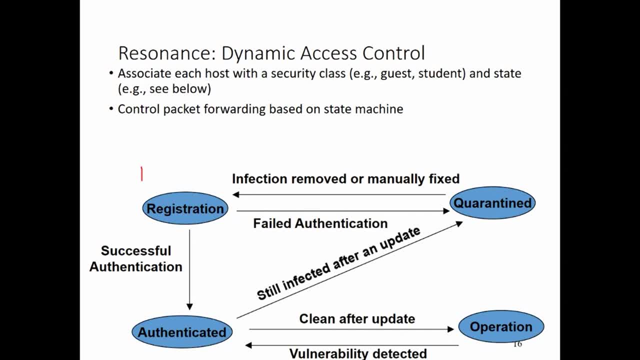 So the first phase is the registration phase And after, let's say, requesting the registration phase, each entity should provide an authentication way. So the second phase is authentication And then, if this client is authenticated, they can do the authentication, And then, if this client is not authenticated, then they will go to a certain zone in the 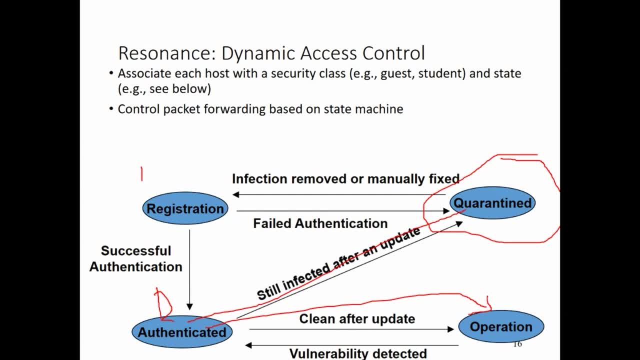 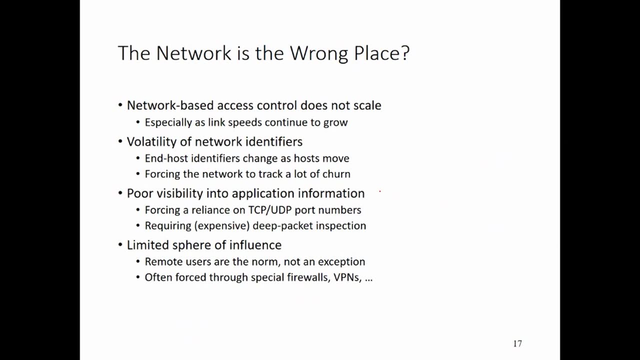 network. It's called a quarantine network, And I'm sure that everybody now know what's quarantine, especially after the many quarantine that we have here in Jordan. Okay, the network is the wrong place, Right? So sometimes- even- That's what for one just mentioned- even if you have the right access, even if you 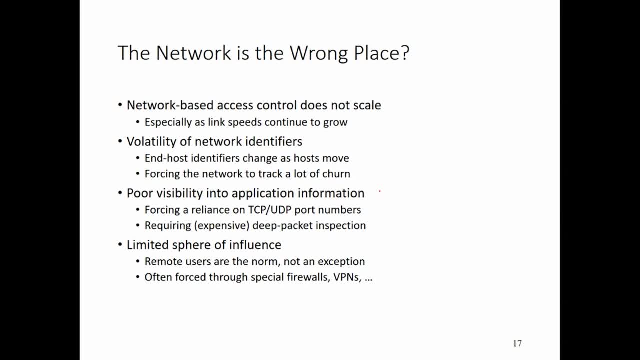 have the right validation or the right authentication information. sometimes you are enforced to go to the wrong network or not the appropriate network that you should use, And that's because of, sometimes, network access, bandwidth Or, let's say, Okay If you have a very poor visibility into some type of application, or because of the congestion. 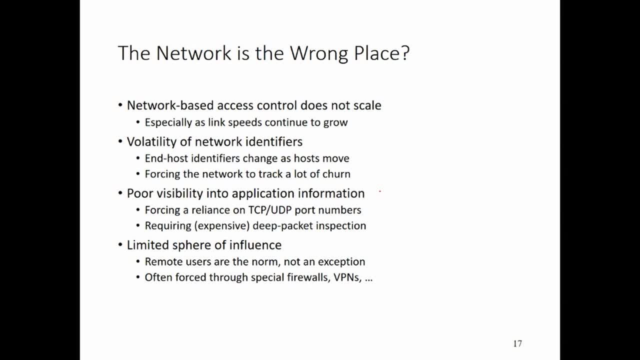 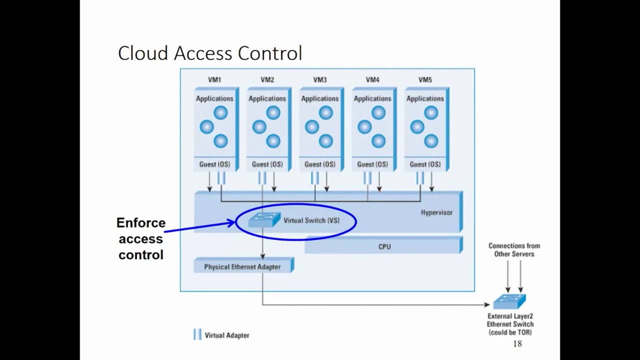 at the firewall or VPNs or even limited sphere of influence based on the remote user and exceptions. We have another type of access control. so we have two types of access control: matrix and dynamic access control, And we have also the cloud access control. 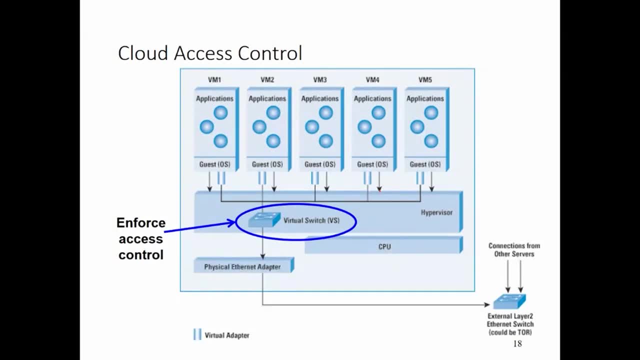 And we use that kind of cloud access control with all the virtual machines. So when Khaled asked you to download the virtual- the Oracle virtual box- and to also install the Kali image on that, so you have a cloud access control installed with the Oracle virtual. 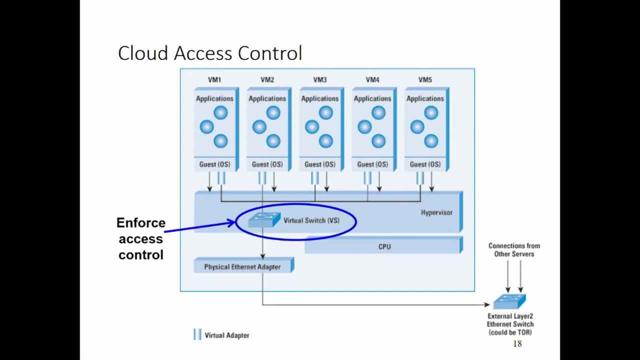 box And, as we mentioned before, If you don't have the agent for a driver, You don't have the agent for a driver, You don't have the agent for a driver. If you don't have the agent for a Dropbox or iCloud or Google Drive, then you can't.